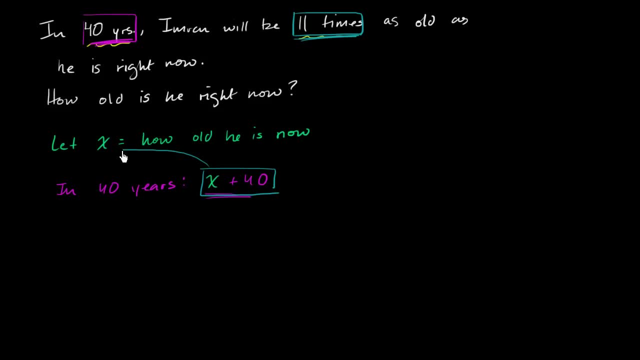 x plus 40, is going to be 11 times as old as he is now. So that's saying that this quantity right over here- x plus 40, is going to be 11 times as old as he is now. So that's saying that this quantity right over here- x plus 40, is going to be 11 times as old as he is now. 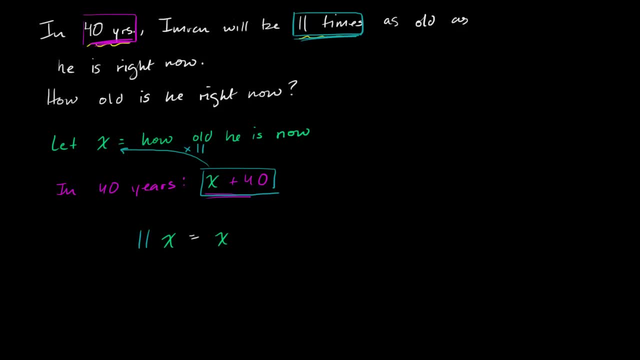 is going to be in 40 years, And we have set up a nice little tidy linear equation now, so we just have to solve for x. So let's get all the x's on the left-hand side. We have more x's here than on the right-hand side. 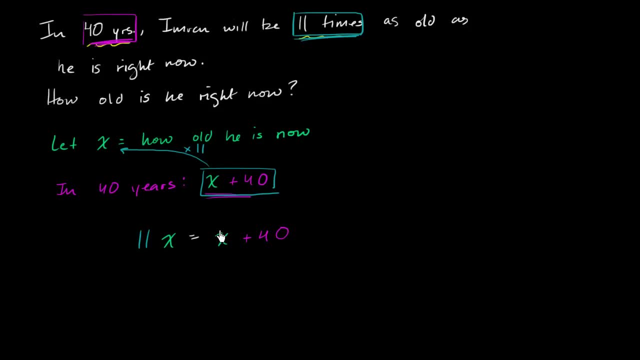 so we avoid negative numbers. Let's take all the x's here. So if I want to get rid of this x on the right-hand side, I'd want to subtract an x, But obviously I can't just do it to the right. 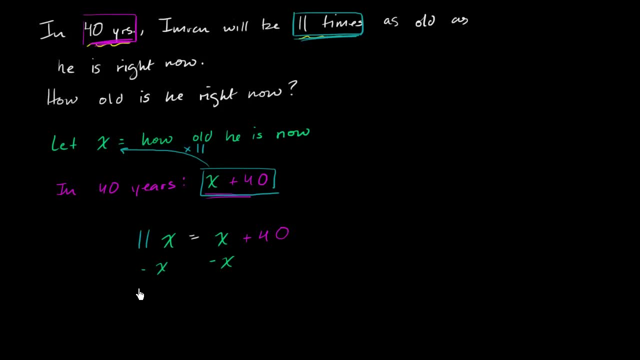 Otherwise the equality won't be true anymore. I need to do it on the left as well, And so I am left with 11.. If I have 11 of something and I take away one of them, I'm left with 10 of that something. 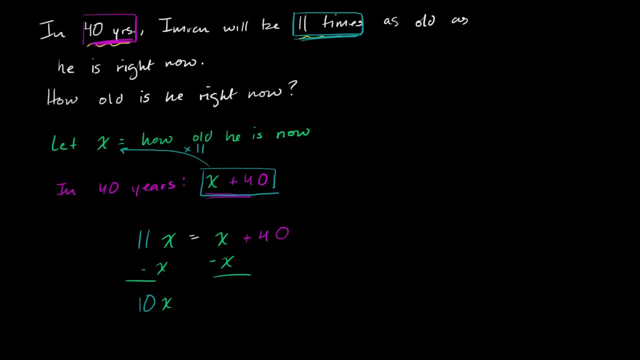 So I'm left with 10 times x is equal to well, these x's, x minus x is just 0.. That was the whole point. It's going to be equal to 40.. And you could do this in your head at this point. 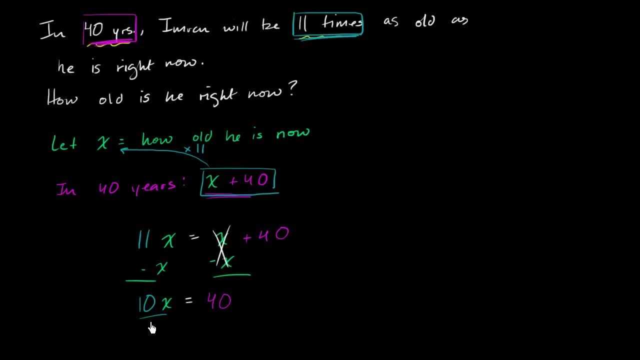 but let's just solve it formally. So if we want a 1 coefficient here, we'd want to divide by 10, but we've got to do that to both sides, And so we are. We are left with, and we can have our drum roll now. 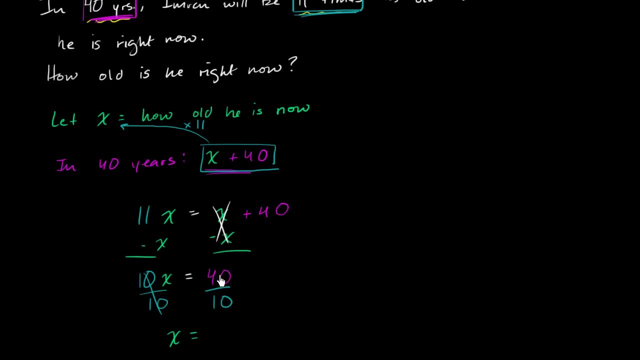 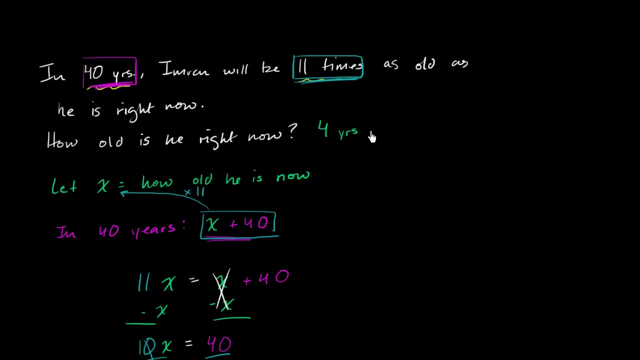 we are left with. x is equal to 4 years old, x is equal to 4.. So I'll answer the question: how old is Imran right now? He is 4 years old, And let's verify this. If he's 4 years old right now, in 40 years he's going to be 44.. 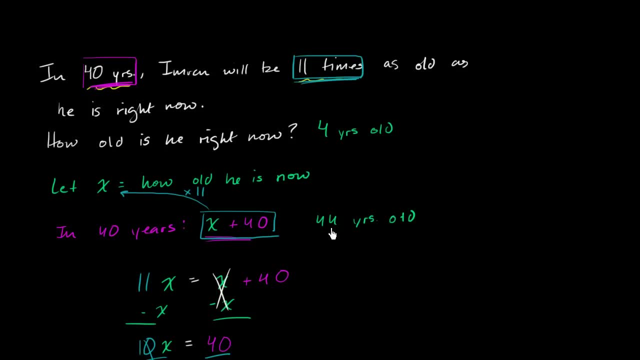 44 years old, And 44 years old is indeed 11 times older than 4 years old. You definitely this is a factor of 11 here. So it all worked out.